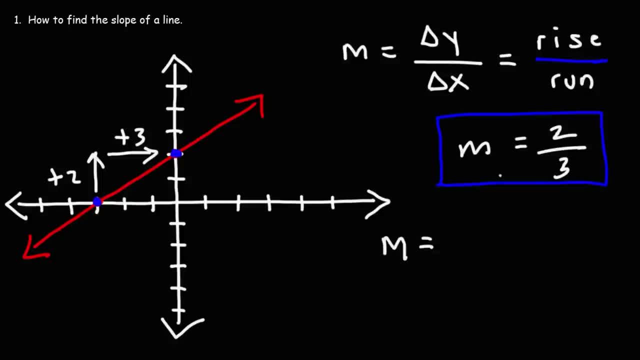 and use this formula: m is equal to the change in y, which is y2 minus y1, divided by the change in x, which is the difference in x values, x2 minus x1.. Okay, so this point here, that's the y-intercept. It has an x value of 0 and a y value of 2.. 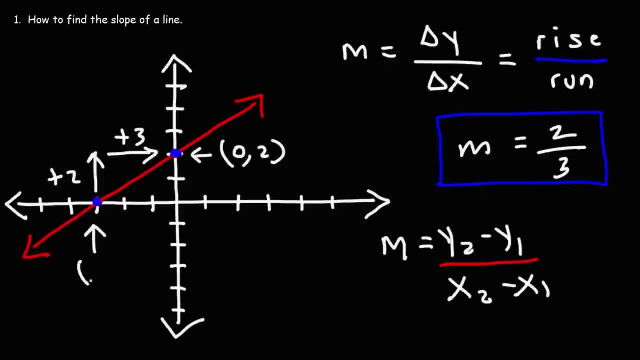 This point here is the x-intercept. It has an x value of negative 3 and a y value of 0. Now let's call this x1 and y1, and for the second point, this is going to be x2 and y2.. So now let's plug in those numbers into this formula. 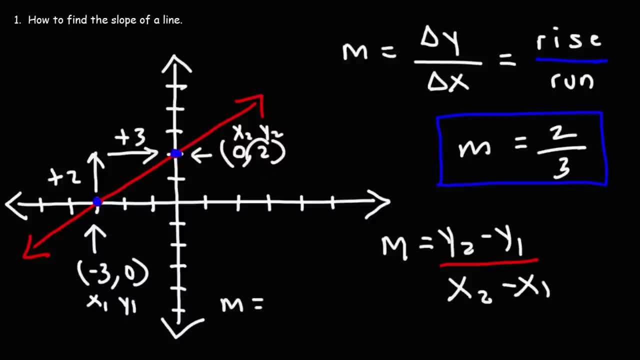 y2 is 2, y1 is 0, x2 is 0, minus x1, which is negative, 3. So the change in y, which is y2 minus y1, that's 2 minus 0, which is 2, and the change in x or 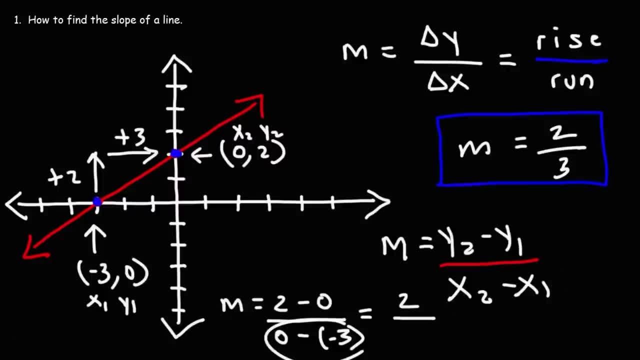 x2 minus x1, that's negative 3.. 0 minus negative 3. Whenever you have two negative signs next to each other, it's going to become positive. So it's 0 plus 3, which is 3.. And so notice that we get the same answer: 2 over 3.. 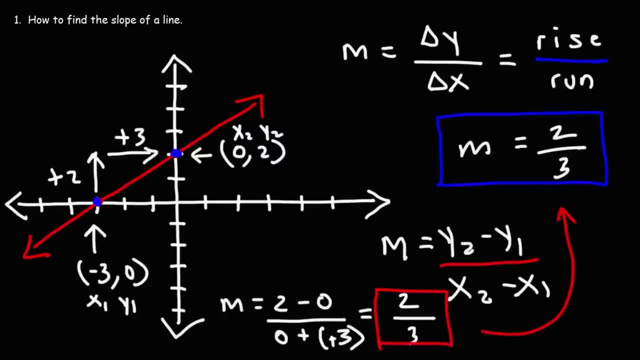 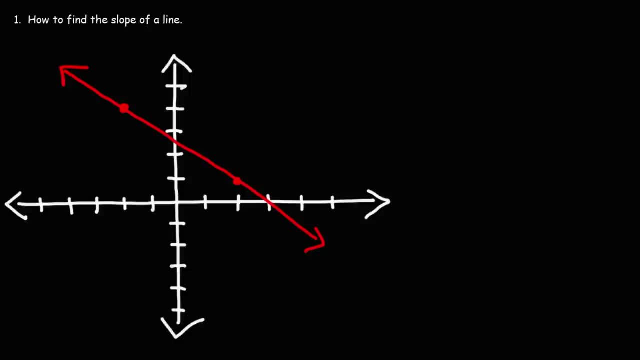 So those are two ways that you can employ to calculate the slope of a line. Now let's try another example. So go ahead and pause the video and find the slope of this line. So the first thing we need to do is choose two points, And we have two points already. 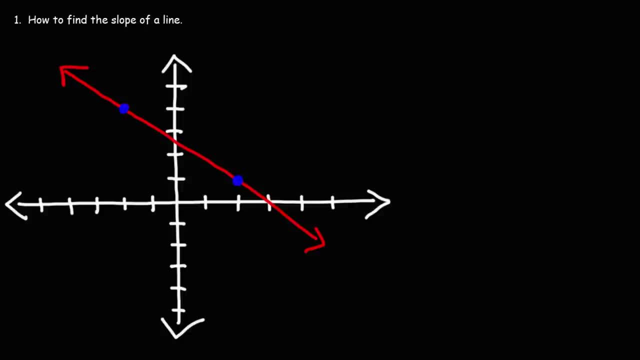 highlighted for us. Now, using these two points, let's find the slope of the line. So let's calculate it by using the rise over run method. Starting from this point and going to the second point, we need to travel down three units, So we have a rise of negative 3.. Now we got to move from left to right and travel. 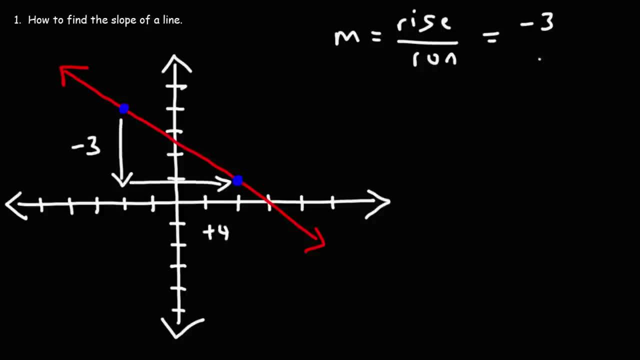 four units to get to the second point. So we have a run of positive 4.. So the slope is going to be negative 3 over 4.. Now let's confirm it with the second method. So we're going to use the formula y2 minus y1.. 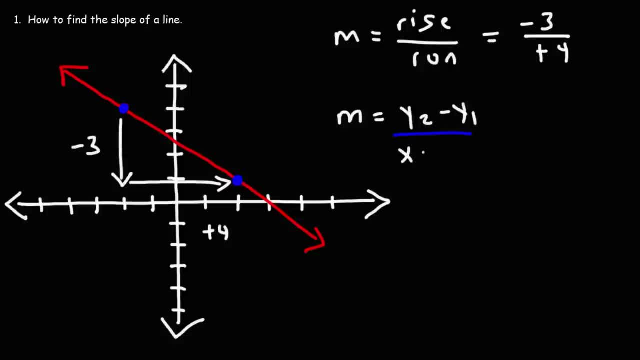 So we're going to use the formula y2 minus y1 divided by x2 minus x1. So this point here has an x value of negative 2 and a y value of not 5 but 4.. Now this other point on the right. it has an x value of 2 and a y value of 1.. 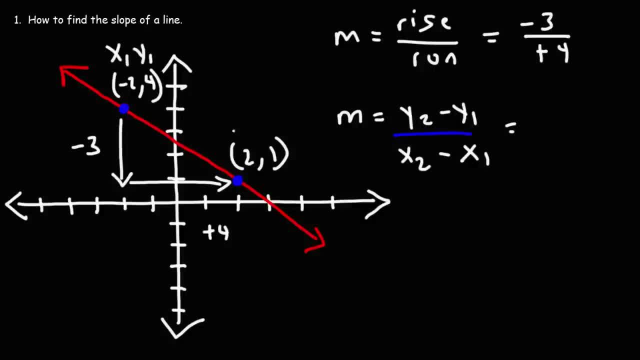 So this is going to be x1, y1, and then x2, y2.. It really doesn't matter which one you label as x1, y1. The answer will still be the same in the end. Now, y1 is I mean, y2 is 1, y1 is 4, x2 is 2 minus x1, which is negative 2.. 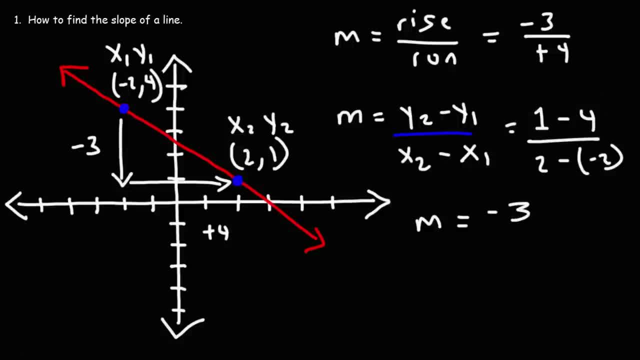 1 minus 4, that's negative 3.. 1 minus 4, that's negative 3.. 1 minus 4, that's negative 3.. 2 minus negative 2, that's the same as 2 plus 2, which gives us 4.. 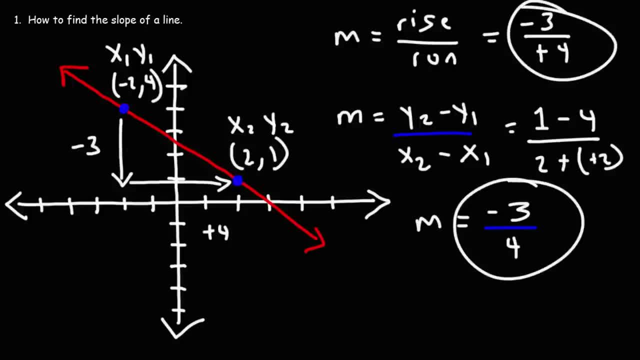 So we get the same answer: negative, 3 over 4.. So those are two ways that you could use to find the slope of a line, But this one is a lot easier once you get the hang of it. Try this one: Go ahead and find the slope of the two lines that you see in this graph. 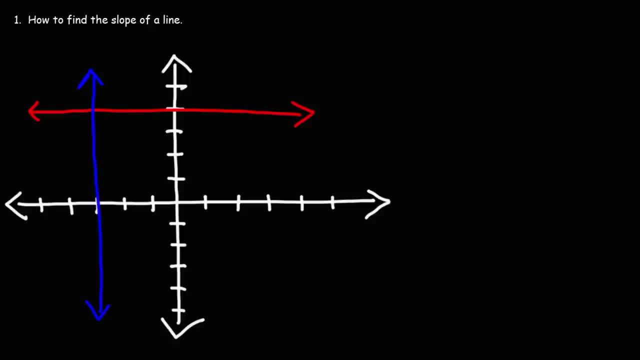 The red line and the blue line. The red line is a horizontal line And the slope of any horizontal line is always 0.. The blue line is a vertical line. The slope for any vertical line is undefined. Now let's talk about why that's the case. 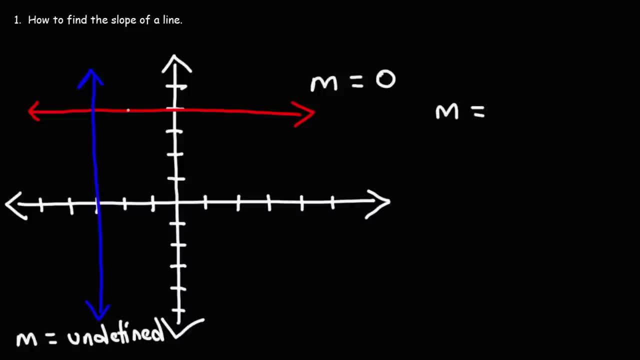 So you can see that the slope of any vertical line is undefined. So you can see that the slope of any vertical line is undefined. So you can see that the slope of any vertical line is undefined. So, using rise over run, if you were to highlight two points on the horizontal line, 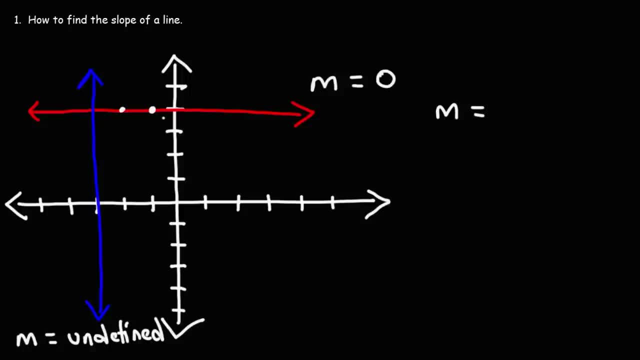 to go from the first point to the second point. you're not going up or down. There is no rise, So the rise is 0.. The run it can vary. It could be, in this case it's only 1.. 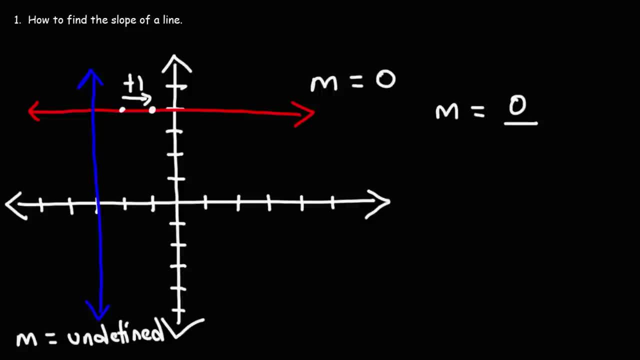 If you choose two other points, the run could be 2,, 3,, 4, 5.. It really doesn't matter what the run is, Because 0 divided by any number is always 0. And so the slope for any horizontal line will always be 0. 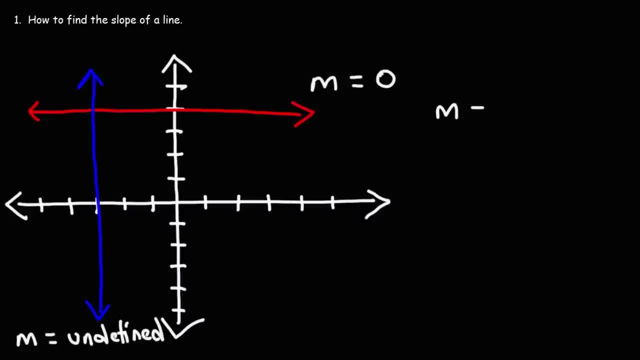 Even if you were to use the other method. So let's say, if we pick these two points, This point here is 1, 4. And the other point is 3, 4.. Let's say this is 5.. So using the formula y2 minus y1,. 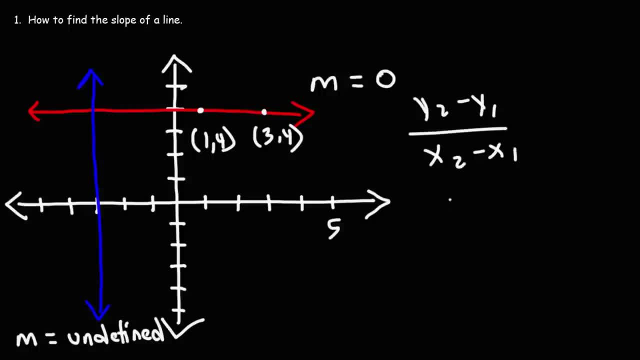 over x2 minus x1.. y2 is going to be 4.. y1 is 4.. x2 is 3.. x1 is 1.. So notice that for a horizontal line, y2 and y1 will always be the same. 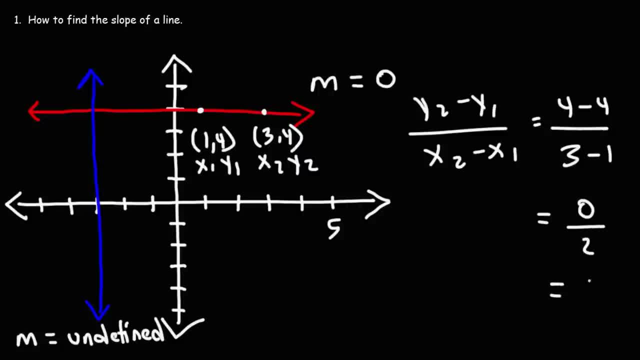 Therefore, you get a rise of 0. And so the slope is going to be 0. So keep that in mind. The slope for any horizontal line? it's always 0.. Now, what about for a vertical line? What is the slope for a vertical line? 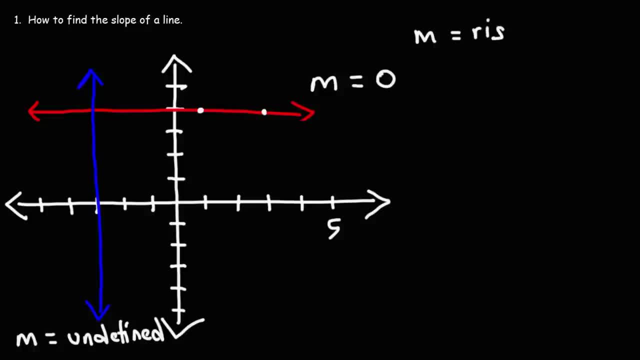 Now, going back to a horizontal line, the reason why the slope is 0, is because the run- I mean the rise- is always 0. That's the case for the horizontal line, For the vertical line, the blue line. this time the run is going to be 0.. 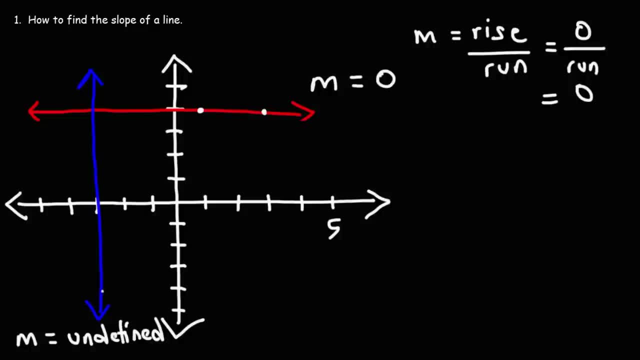 Not the rise but the run. So if we pick two points, let's choose these two points. Notice that we have a rise of positive 2. But because, to get to the second point, you're not moving to the left or to the right. 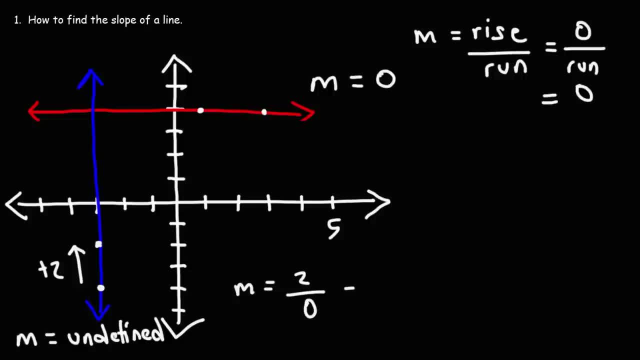 You're just going straight up. The run is 0. And whenever you have a 0 in the denominator of a fraction, the value is undefined: 2 divided by 0, we don't know what the value of that is.